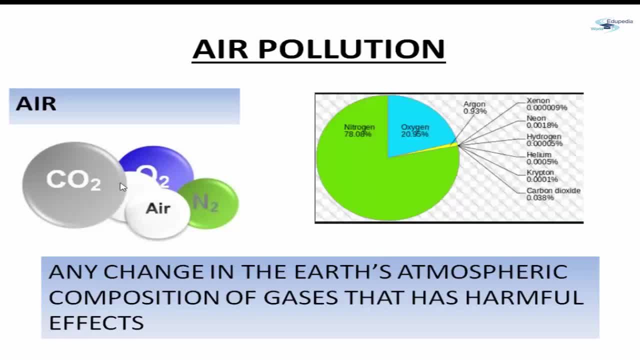 right. So that is what is air, If there's any change in this composition. like what is the composition? The composition as you see here: nitrogen is 78.08% and oxygen is 20.95%- right, And the rest of it, which is very, very less in quantity, it includes other trace gases. 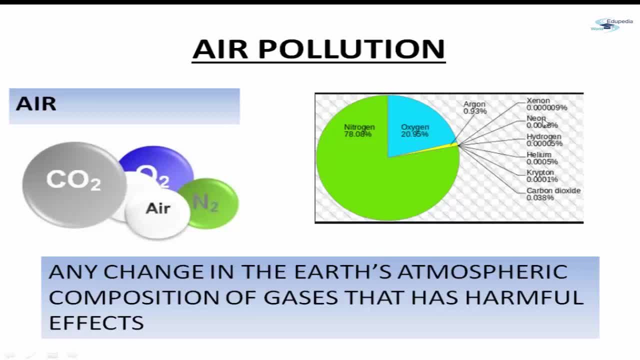 as I said, like argon, xenon, neon, hydrogen, helium, krypton and carbon dioxide. So these are the other trace gases. So what is air pollution, In case there is any change in this atmospheric composition of gases that has harmful effect on the environment or on the 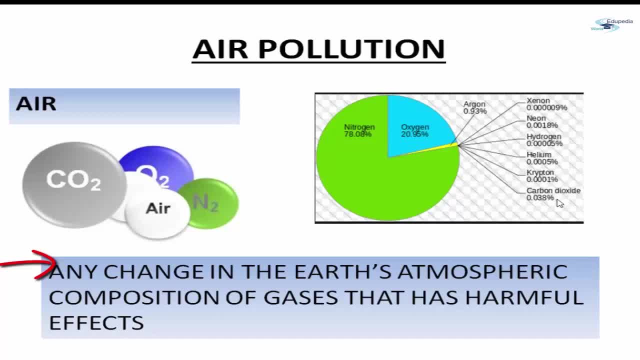 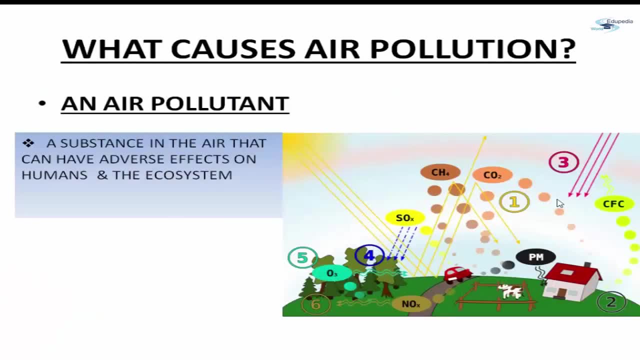 human beings or on the wildlife or the surrounding. it is known as air pollution. Now, what causes this air pollution? Air pollution is caused due to air pollutant. Air pollutant is something which pollutes the air. So what is this air pollutant? An air pollutant is a substance. 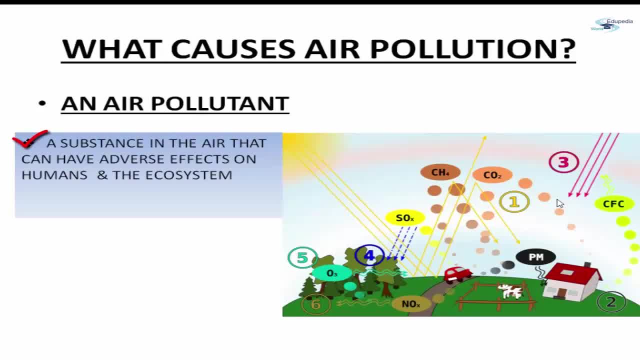 in the air have very, very adverse effect on the humans and on the ecosystem. that is what is called as a pollutant, and pollutant can be anything. it can be methane, it can be the co2, which is the carbon dioxide. it can be the chlorofluorocarbons, the 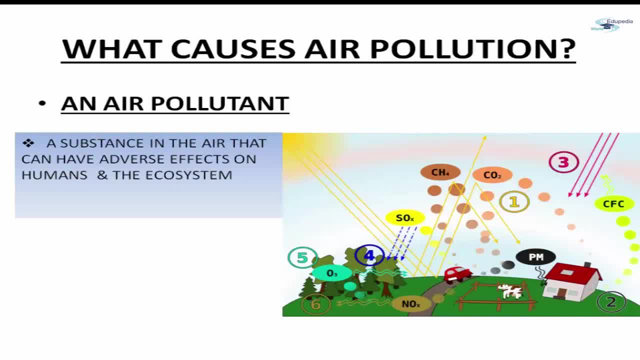 nitrogen oxides, the sulfur dioxide, which is generally comes out of the industries. so that is what is known as a pollutant. the substance that is the pollutant can be solid, it can be liquid, it can be in a form of, you know, gases also, and this 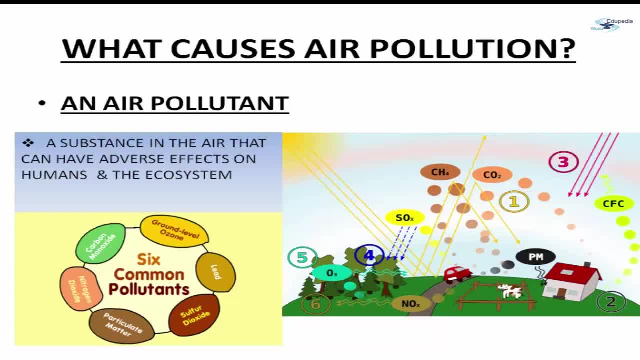 pollutant can be either natural pollutant or it is. it can be man-made pollutant, that is, it can be naturally produced or it can be man-made. right, but first of all, what are the six common pollutant? the six common pollutant are, as flashed here: the ground level ozone, the lead, sulfur dioxide particulate. 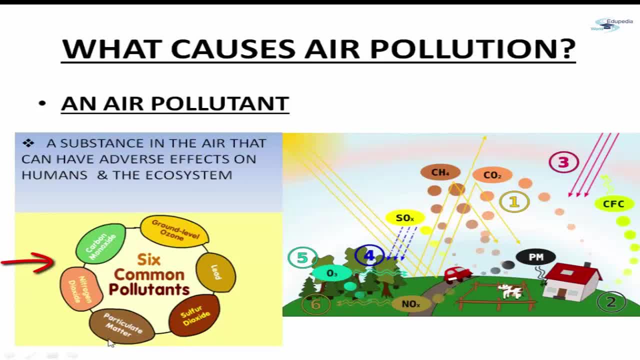 matter. these are very, very fine particles: nitrogen dioxide and carbon monoxide. carbon monoxide is also caused because of burning of fossil fuels. so these are six major, very, very common pollutant that we find in the surrounding. so, as I said, a pollutant can be solid liquid gases, it can be man-made or natural. so 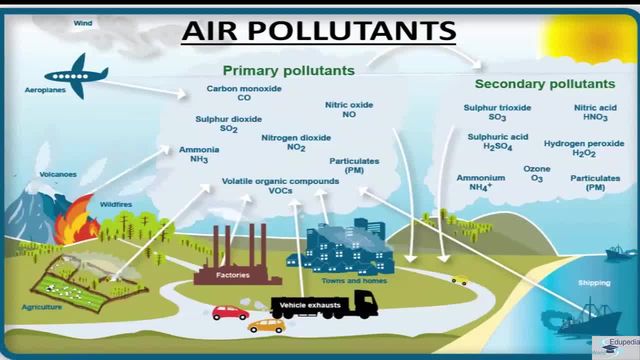 these are various categories of a pollutant. so this is what is shown to you here is the primary pollutant and the secondary pollutant, because, as I said, pollutant can be of two types: primary and secondary pollutant. what is primary pollutant? primary pollutant are usually produced from a process such as: 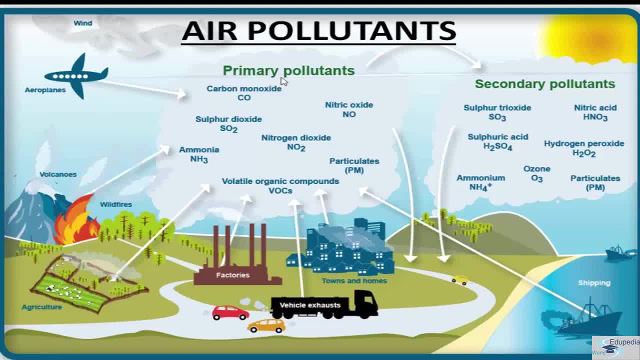 an ash from a volcanic eruption. other examples of primary pollution includes the carbon monoxide gas which comes out of the vehicle exhaust, the sulfur dioxide which is released from the factories, whereas, on the other hand, the secondary pollutant are basically the pollutant which are not emitted directly from the environment. rather, they form in. 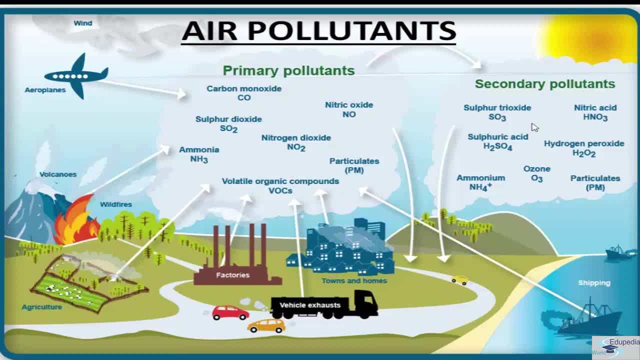 the air when primary pollutants react or they interact with some other pollutant right, so that those are called as secondary pollutant. these secondary pollutant, in other words, we can say that they are produced from the primary pollutants. so in other words, they are produced from the primary pollutants. so in other 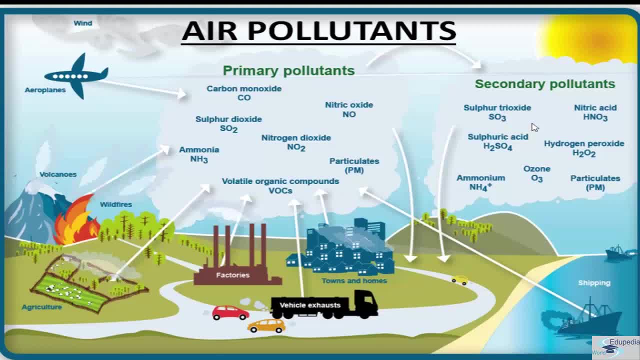 words, we can say that the secondary pollutants are the ones which are formed because of primary pollutant or from the primary pollutant. what are the other examples of secondary pollutant? is like nitric acid, hydrogen peroxide, particulate matter, the O3, which is the ozone ammonium. 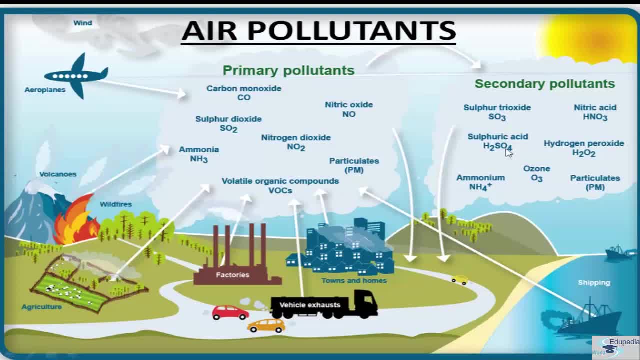 sulfuric acid. so these are all the secondary pollutant which are generally caused because the primary pollutants keep interacting with each other. okay, one thing that you should note here is that they may be pollutants which may be both primary as well as secondary pollutant, so they may 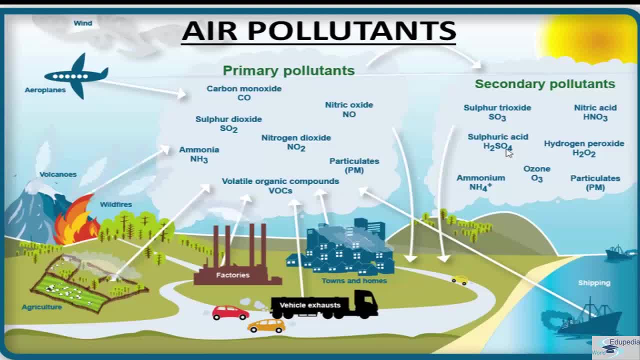 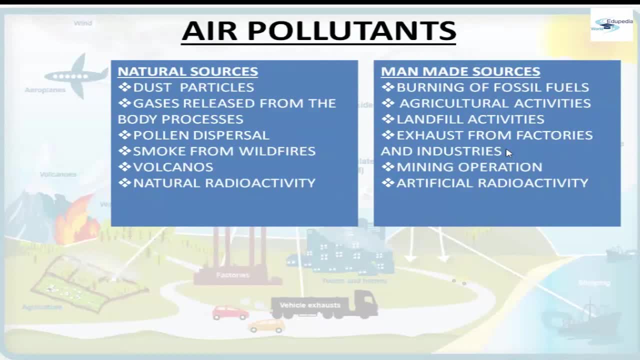 fall under any of the category, or even both the categories. we talked about primary and secondary pollutant. let's now talk about some of the natural sources and some of the man-made sources. these are natural pollutant and man-made pollutants. so the natural pollutants will consist of dust particles. 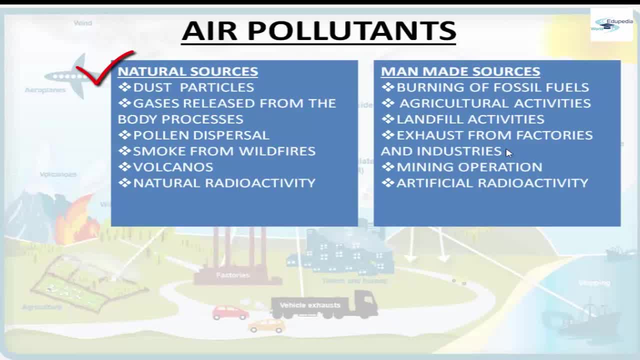 gases which are released from the body processes, pollen dispersal, smoke from the wildfires, volcanoes and natural radioactivity. on the other hand, the man-made sources are produced from burning of the fossil. then you have the agricultural activity, landfills, exhaust from the factories, mining operations and artificial radioactivity. right? so these are some of the 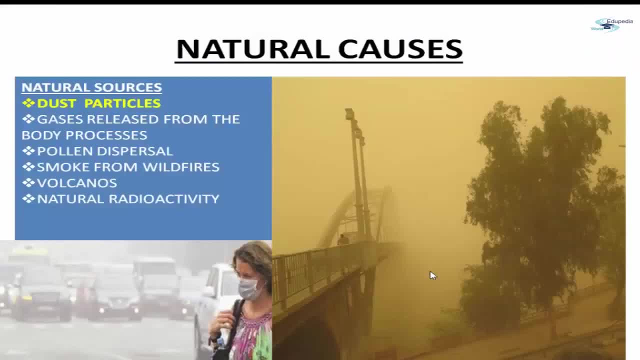 the natural and some of the man-made sources. so let's now talk about the natural causes, how these natural pollutants are produced. so first is dust particles. so dust particles, it is very, very commonly you must have seen that whenever the wind blows with a faster speed it actually throws all the dust up in the air from the ground, so that actually pollutes the. 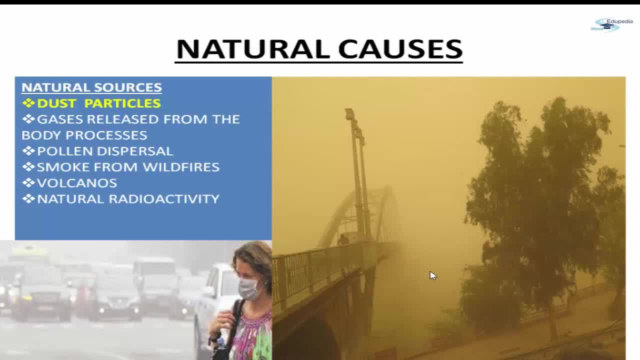 environment. so this is, this is what is what are known as a dust particles, and lot of people have severe respiratory problems due to these dust particles. so you see here this lady. she's covering her mouth and her nose. that is just to avoid any kind of dust particles. right next is gases. 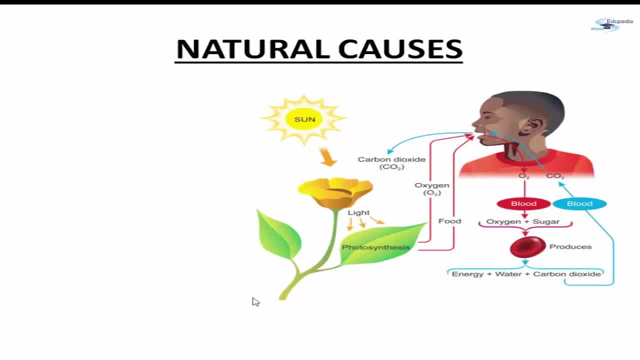 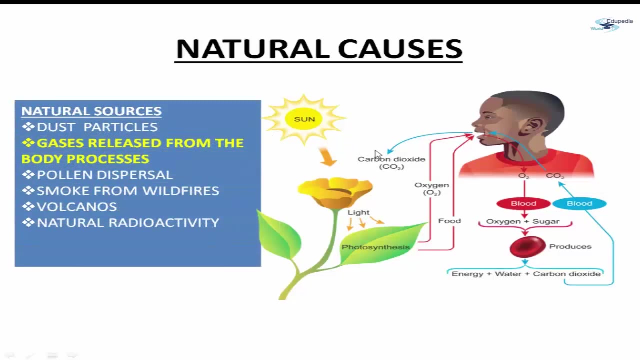 released from the body processes. what are these gases which are released and how are these gases released? the gases are nothing but the carbon dioxide is released from the human body. basically, when we breathe, the co2 comes out and the oxygen is taken inside, and that co2, what comes out, is used by the plants in order to you know. 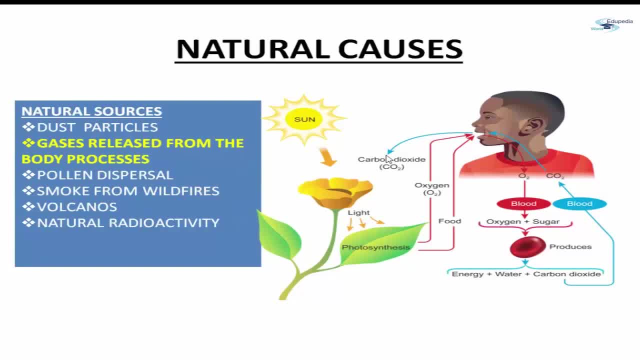 prepare their food and to carry out the process of photosynthesis. so that's how this is. the entire process goes in, carbon dioxide goes out. when the carbon dioxide goes out, it is a kind of pollution. so the more the number of population, the more carbon dioxide will be produced, right? so this is. 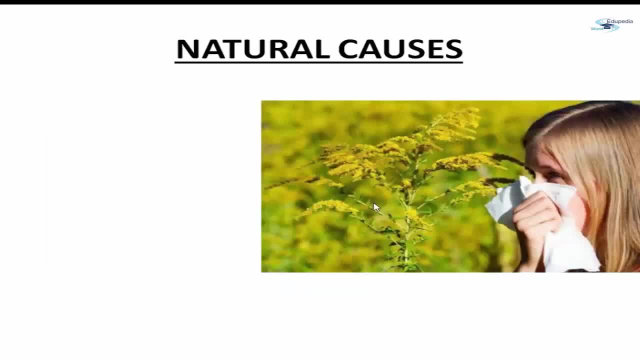 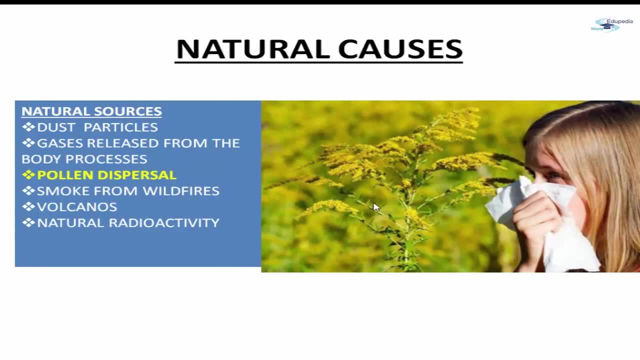 a natural pollutant. next are the pollen. pollens are also some of the natural pollutant pollens: from grasses, from trees, from weeds. these are wonderful substances because they allow plants to reproduce. but pollens are found to be naturally available in the air, but now, because of the 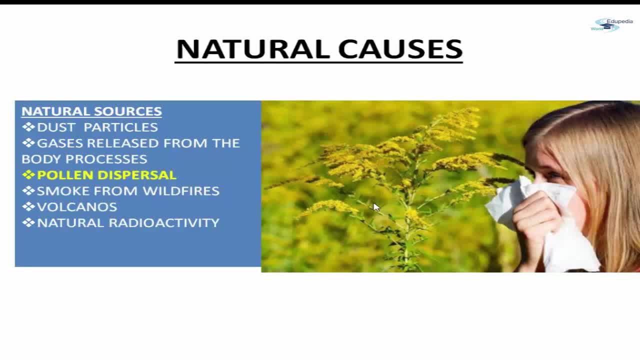 activities of human beings and other animals and birds. these activities, the pollen activities, also further increases in the air and these pollens can actually cause a lot of allergic problems and a lot of less respiratory problems among the human beings. especially the childrens are also prone to. 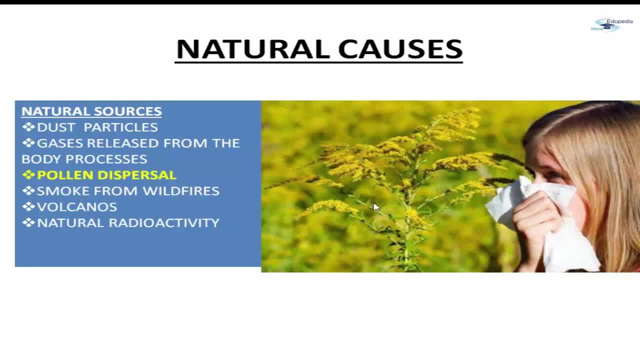 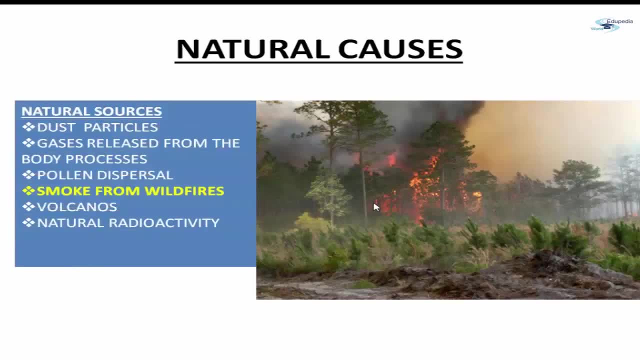 such allergies from the pollens. so the pollen dispersal is also a natural way of causing the air pollution. next is smoke from wildfires in the the forest. they automatically catches fire during the summer season and this fire creates a lot of black smoke that you can see is coming out. 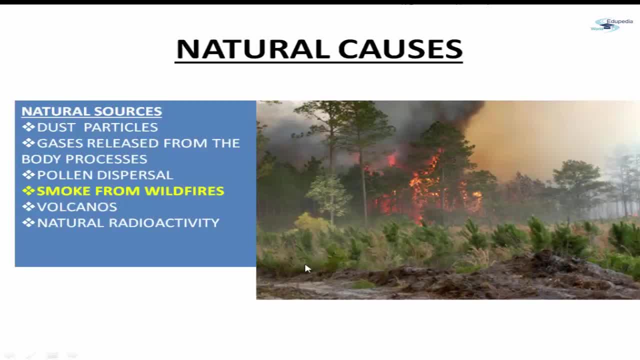 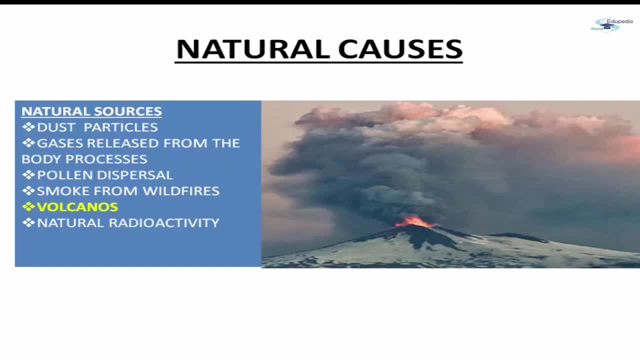 from the fire, and this is a natural pollutant- volcanoes. volcanoes also cause a lot of pollution. what comes out from the volcano is called as magma, so magma contains a lot of dissolved gases, which provides a driving force that causes most of the volcanic eruptions. now, even if the magma doesn't reach the surface, let's say it is just below the surface. 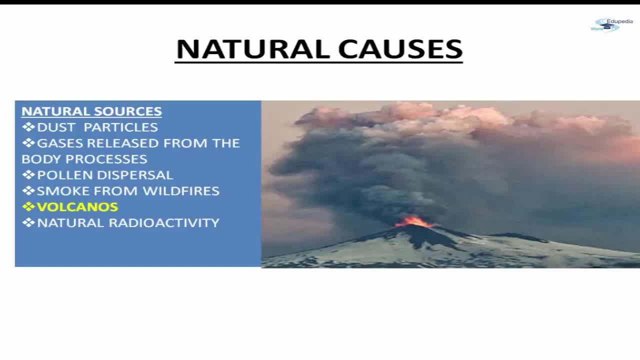 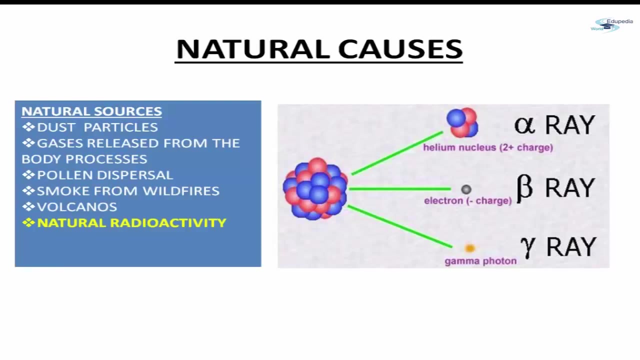 even then, those harmful gases are released in the atmosphere through that smoke which is coming out. this can pose a very, very serious risks to people and animal and the other wildlife. these harmful gases can lead to headache, dizziness, increased heart rate and difficulty in breathing. so natural radioactivity is also a natural pollutant. natural radioactivity is seen generally. 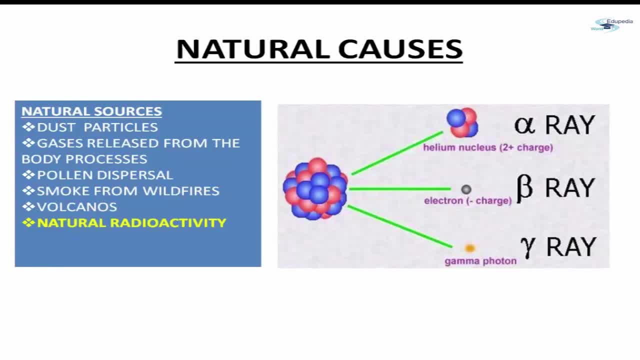 in the rocks and in mountains, and it takes place continuously- those rocks and soil we are using in order to build our houses. so this natural radioactivity also releases the three particles of the air, as well as the three molecules like the alpha, the beta and the gamma. these particles are not again. 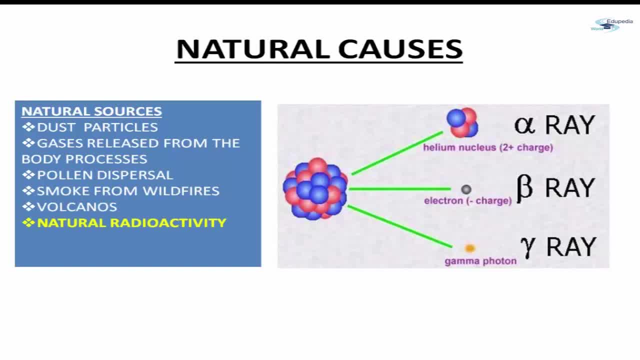 healthy for our human body. so that is why even natural radioactivity is also very, very harmful. so these are some of the natural causes through which the natural pollutants are produced and they pollute the air and they cause air pollution. now let us have a look at some of the man-made activity. 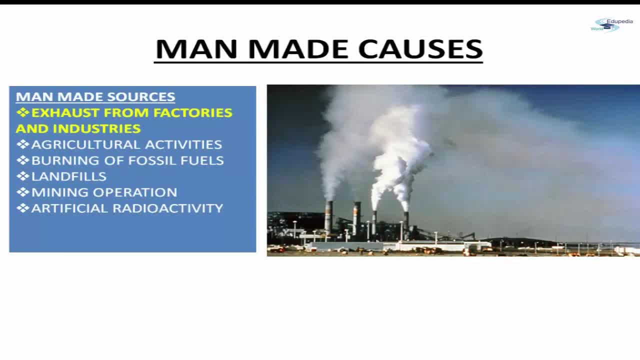 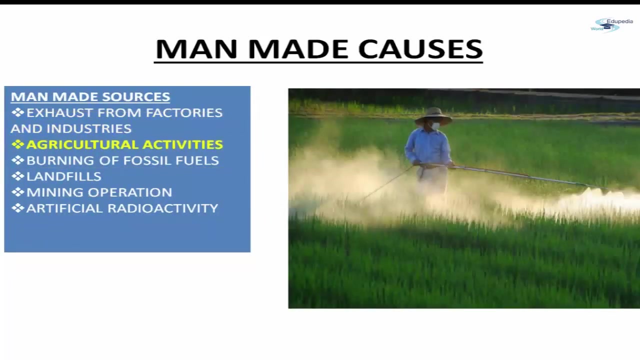 includes the exhaust from the factories and industries. these industries produce smoke as a main pollutant. the smoke comes out of the industry and this smoke contaminates the air. it contains a lot of toxics. it contaminates the air by releasing those toxic gases in the air. next is the agricultural activities. how? 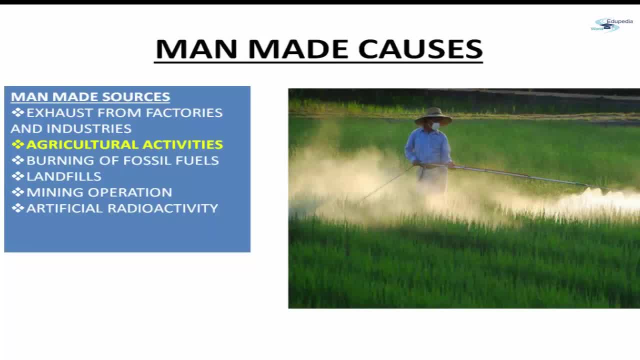 can agriculture create pollutants which are man-made? in addition to methane and nitrogen oxide, agricultural activity has also been linked with the emission of some of the dangerous gases and pollutants. and what are these gases and pollutants? these include carbon dioxide, ammonia, hydrogen sulphide and airborne particulate matter. so that way from the agricultural activities. 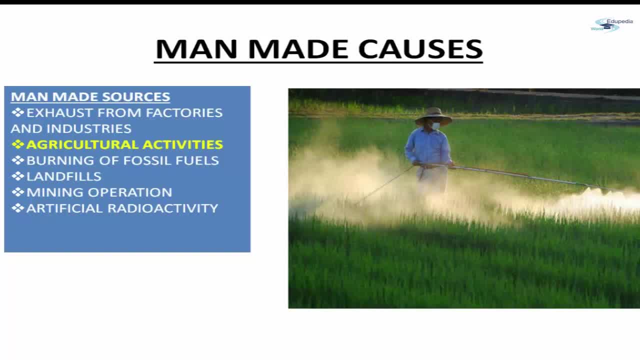 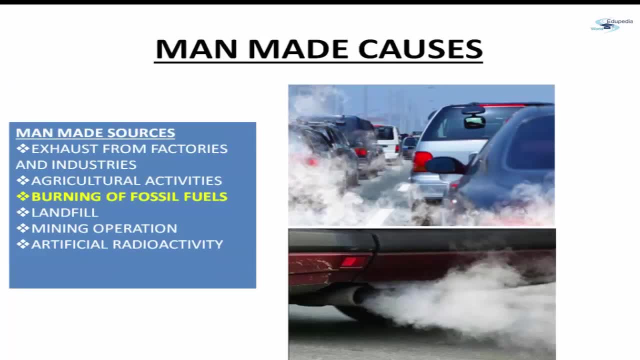 are created a lot of toxic gases and pollutants which are man-made and, as I said, these are man-made so that way from the agricultural activities are created a lot. also, there are some harmful gases which are released which are not good for humans. Next is burning of fossil fuel. These days you must have seen the cars and the heavy. 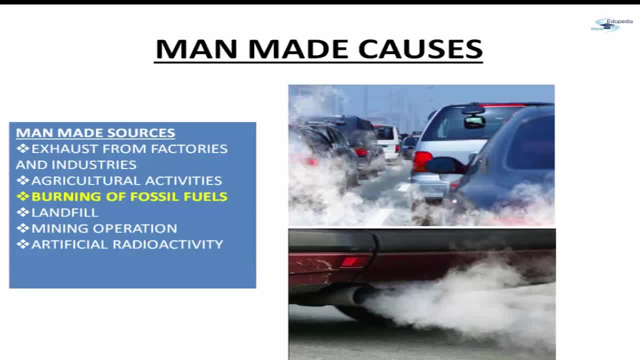 duty trucks and trains and aeroplane. They all burn a lot of fossil fuel. You can see a lot of smoke on the roads coming out from these four wheelers and two wheelers, And this emission from the automobiles includes both primary as well as secondary pollutant, And this is a major cause. 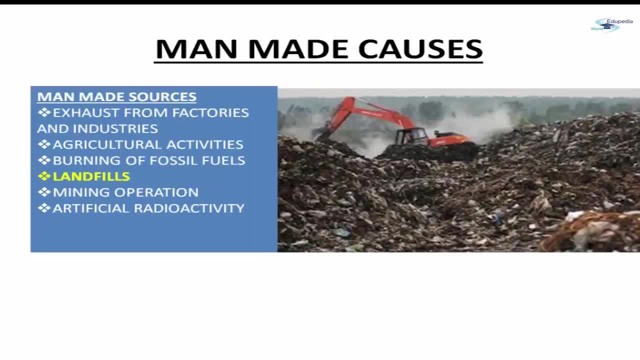 of pollution these days, of air pollution Landfills. Landfills are again another man-made source of pollution which creates a lot of air pollution. There are over 10 toxic gases that are released from any landfill, Of the most serious of which is methane, So methane is the most. 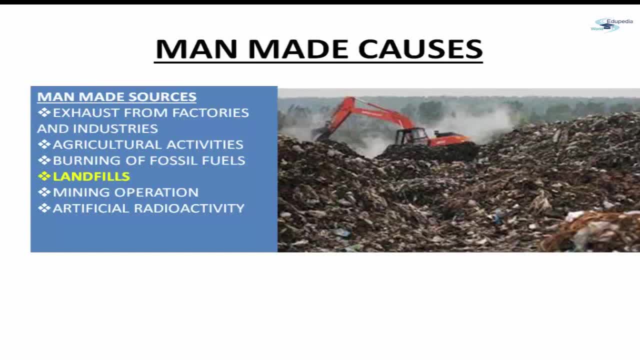 dangerous gas. Methane gas is naturally produced during the process of the decay of any organic matter, And this methane is more potent greenhouse gas than the carbon dioxide, So it is very, very dangerous. So as far as possible, the landfills are supposed to be cleared off and a separate dumping ground. 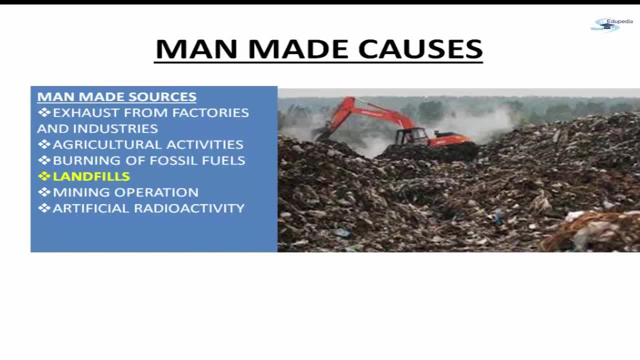 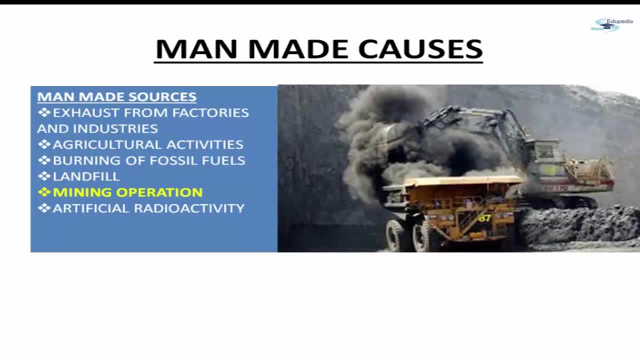 should be created. Landfills should be far from any residential areas. Mining operations: So we talked about mining operations in our previous video, when we were talking about soil pollution. Mining operation creates a lot of soil pollution, But these operations also produce a lot of air. 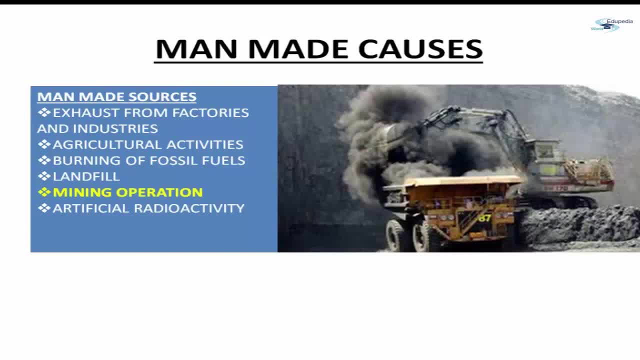 pollution. Mining is a process wherein the minerals are actually extracted from below the earth surface, Are extracted by using huge equipment, So during this process there is lot of dust that is released in the air, which creates massive air pollution, and this is one of the reason which is responsible for deteriorating the health conditions of the 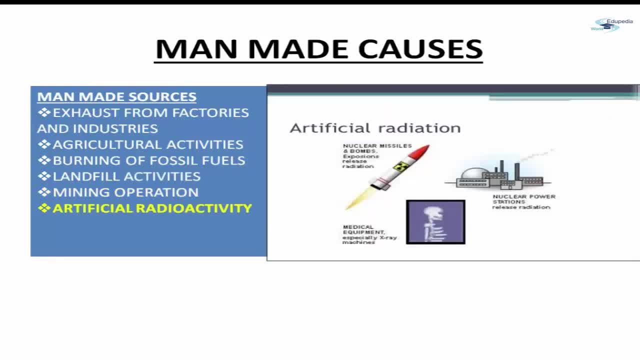 workers and the nearby residents. Last is artificial radioactivity. We talked about natural activity, wherein, naturally, in the rocks and in the soil, the radioactivity is taking place. Artificial radioactivity actually includes mining of any radioactive ore. so when the radioactive ore are mined, lot of harmful gases are again released. The mining of radioactive ores includes: 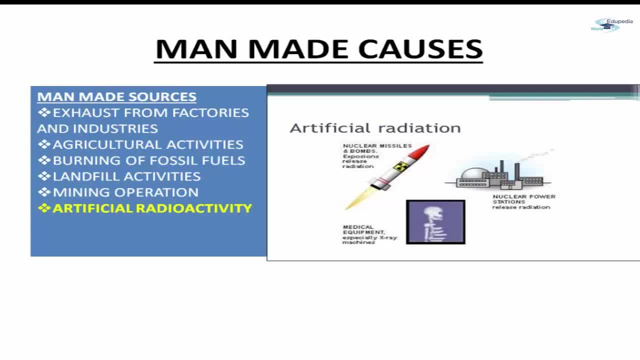 the crushing and the processing of that radioactive core. Secondly, there are other activities, for example the nuclear waste handling and disposal. Whenever there is any nuclear waste, its handling and disposal is very, very important because it may generate low to medium radiations over long. 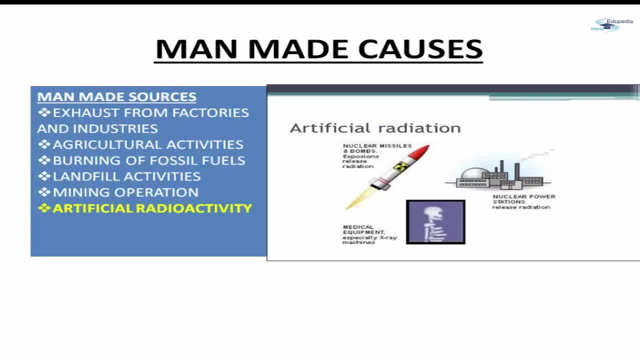 period of time and those radiations are very important. So, for example, if you have a nuclear waste handling and disposal, those radiations are again not good for human beings. Other activities which gives rise to artificial radioactivity is nuclear explosion. Again, if there is any nuclear explosion, lot of. 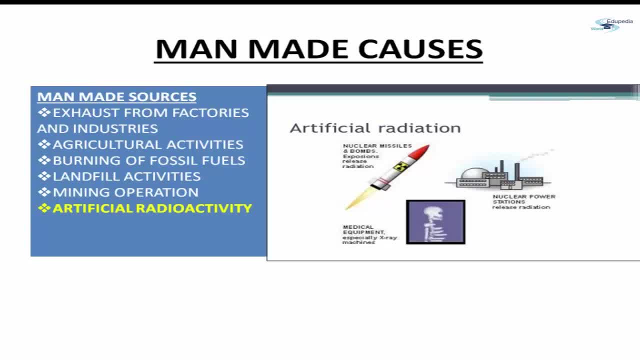 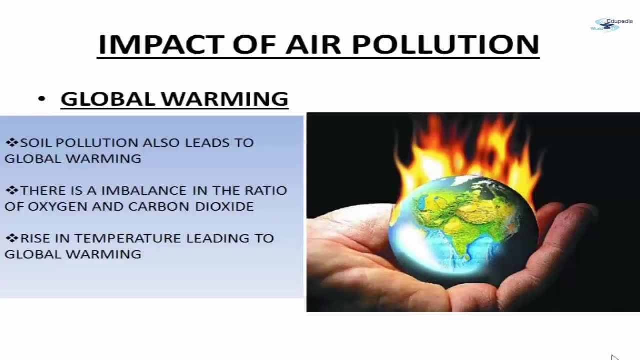 nuclear and radioactive gases are produced, which is not good for the environment, and it also include detonation of nuclear weapons. So that is how artificial radioactivity is not good for the human health. So now that we have discussed the two things, let us move on to the next one, which is the radiation. 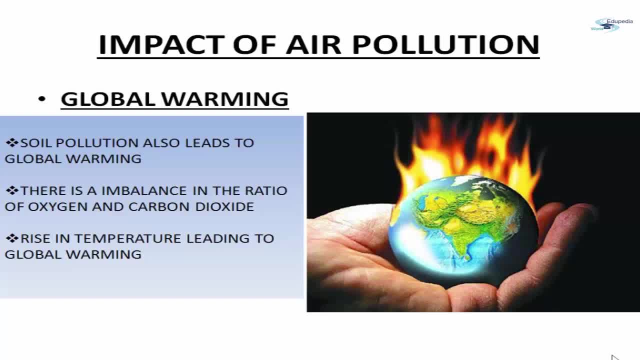 pollutionallocation, where we have talked about natural and man-made sources of air pollution. We spoke about how air pollution is caused And what is pollutant. Let us now talk about impact of air pollution. What happens because of the air pollution? There are health problems that are caused because of air pollution, but then more. 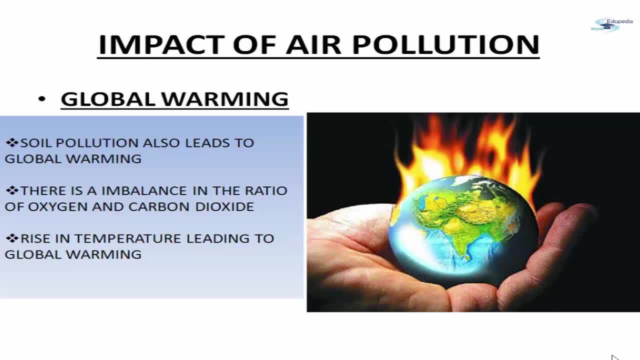 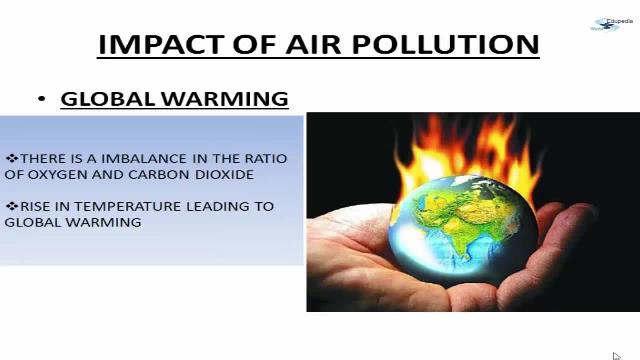 than health problems. also, the entire environment is getting polluted because of air pollution. So let's now talk the impacts of air pollution. So the first impact that we're going to talk about is global warming. What is global warming? Global warming is the rise in the temperature of the air around the 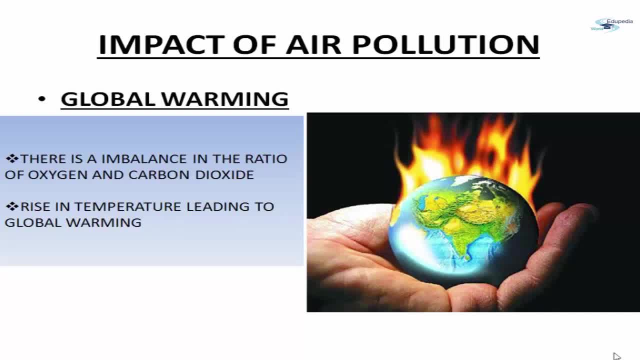 surface of the earth and this rise in the temperature is basically because of the imbalance in the ratio of oxygen and carbon dioxide. Why does this imbalance takes place? Because there is a lot of air pollution, a lot of carbon dioxide is being emitted, and when carbon 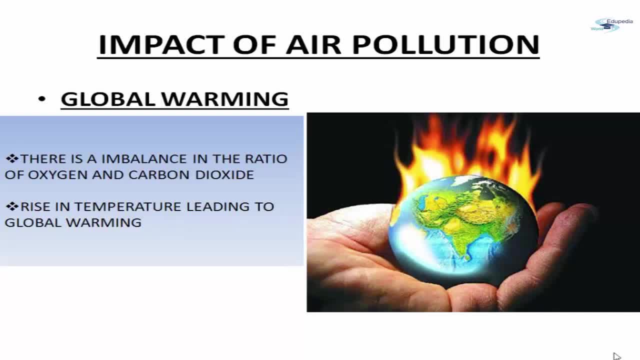 dioxide is more. the ratio between the oxygen and this carbon dioxide is imbalanced. There is a perfect ratio between both the gases and when the air pollution takes place, the CO2 increase. The amount of the CO2 in the environment is more So when the ratio of oxygen and carbon dioxide 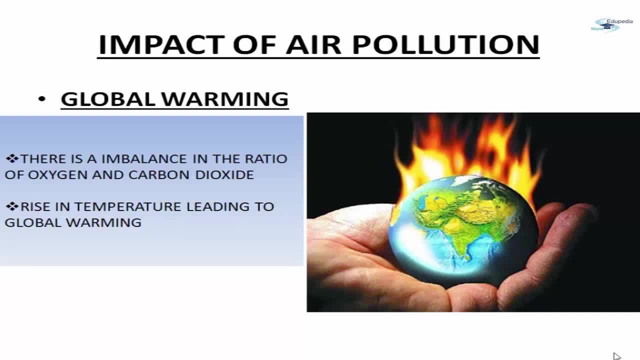 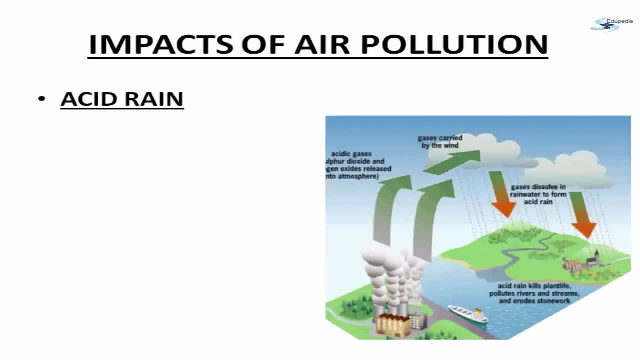 is imbalanced. there is rise in the temperature of the air around the surface of the earth and this gives rise to global warming. So next impact is acid rain. So what is acid rain? Acid drain is the smoke that is coming out of the industries goes up. The smoke contains sulphur dioxide and nitrogen oxide. 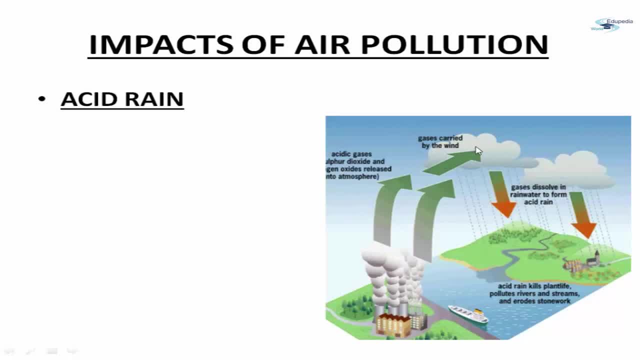 The smoke goes up, forms the clouds and during precipitation, when the rain takes place, this these harmful gases are dissolved in the rain and When it falls on the soil, it pollutes the soil, it pollutes the water and it also pollutes the air. 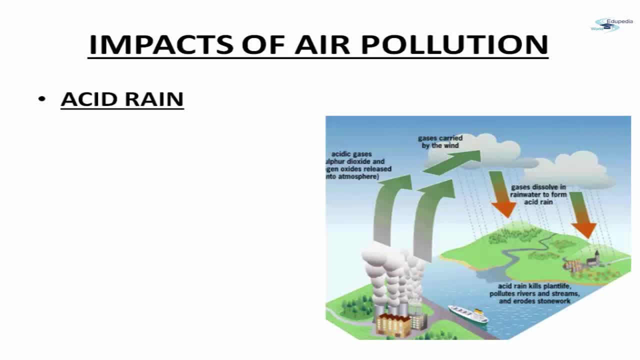 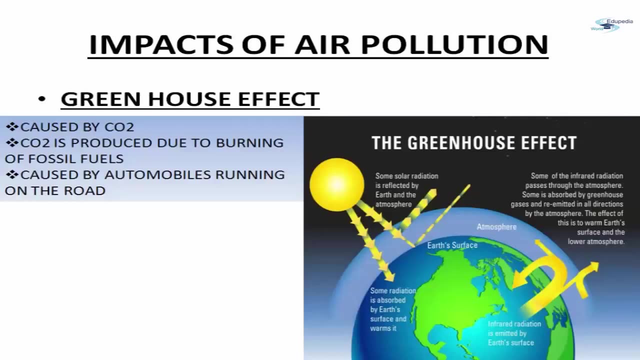 and that's why all the three- the soil, the air and the water- is polluted. So this is known as acid rain, which is not good for the marine life, which is not good for the wildlife and the environment on ground and, of course, the air is polluted. Greenhouse effect is the next impact. 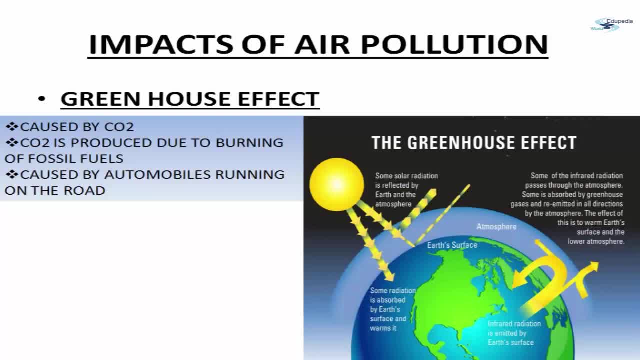 of air pollution. What is greenhouse effect? It is caused because of the carbon dioxide, and this carbon dioxide is produced due to the burning of fossil fuel, Fossil fuel. what I'm talking about is the fuel that is burning in our automobiles, which are running on the road. 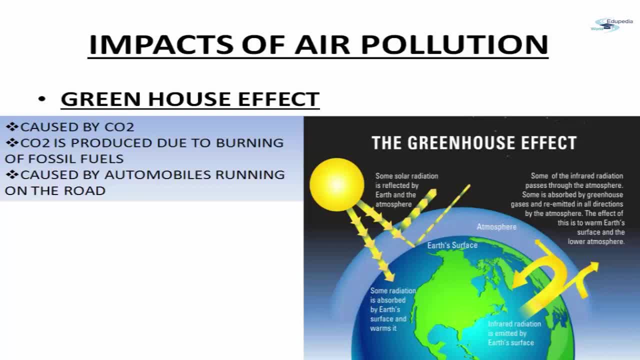 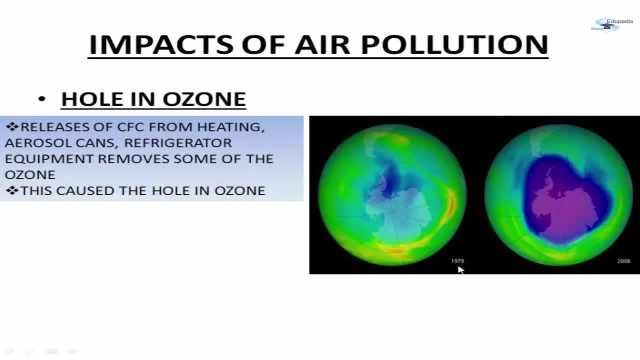 So the more the number of automobiles, the more number of fuel which will be burned and more will be the carbon dioxide. and if the carbon dioxide is more, then it will give rise to CO2.. greenhouse effect. next is hole in ozone. you have two pictures in 1979. you see this blue color shade. 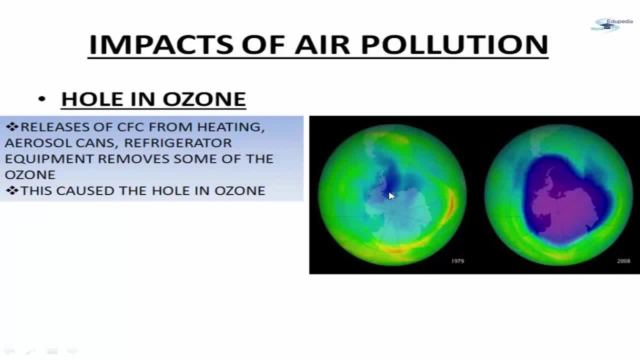 over here shows the depletion of ozone, whereas in 2008 you see so much of ozone depletion has taken place. this ozone depletion- that is, the hole in ozone- is due to the chlorofluorocarbons that are produced from heating the aerosol cans, refrigerators, equipments. so 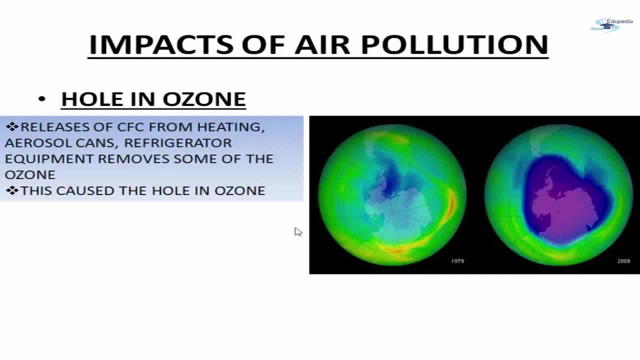 these causes the hole in the ozone. these equipments also causes a lot of air pollution. in case the depletion of ozone continues to take place in the similar way as it has been taking place, so there won't be any ozone layer and those harmful uv rays that are coming from the sun. 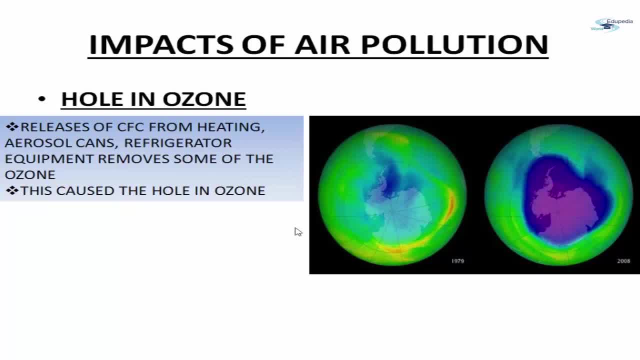 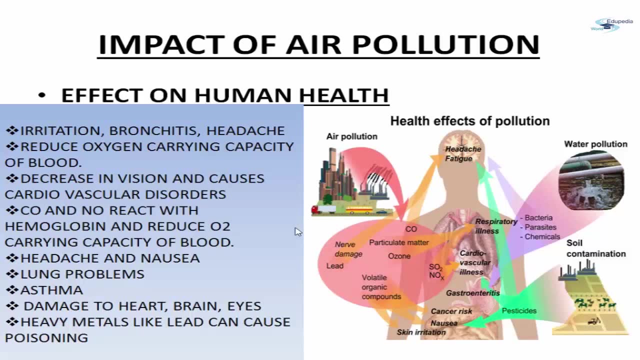 will directly enter the surface of the earth and people have lot of problems, including the skin problems, the problems with the eyes. So hole in the ozone is another impact of air pollution. Biggest effect is on our human health. We have problems including the irritation, the bronchitis, headache, reduced oxygen supply. 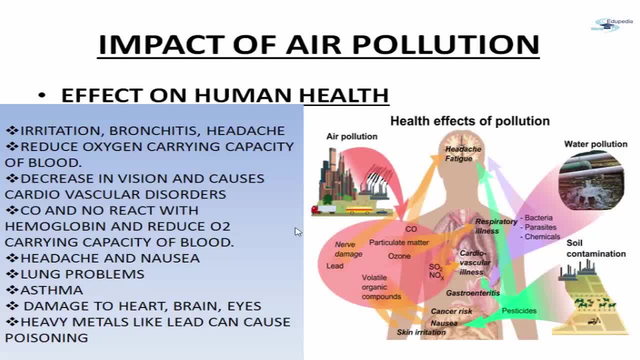 to the blood, then decreased vision, and it also causes some of the cardiovascular diseases. Few other problems are related to lungs. we may have respiratory problems. people, or especially the children, may develop asthma. they may have headache and nausea. the hemoglobin in the blood may drop down. 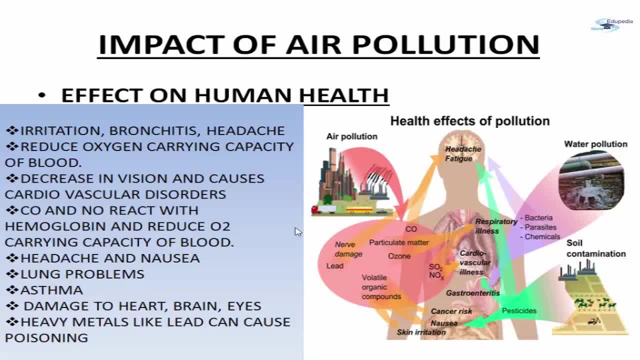 We may suffer from heart problems, problems in the eyes, problems in the brain, and there are some heavy metals, like lead, which can also cause lot of poisoning. So there are n number of problems that are affecting our health, Which is mainly due to air pollution, because air is something that we need. air is something 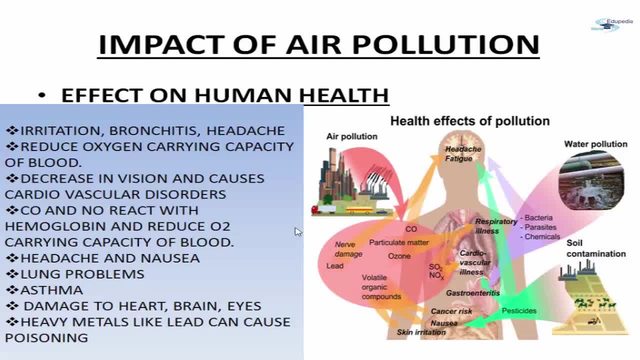 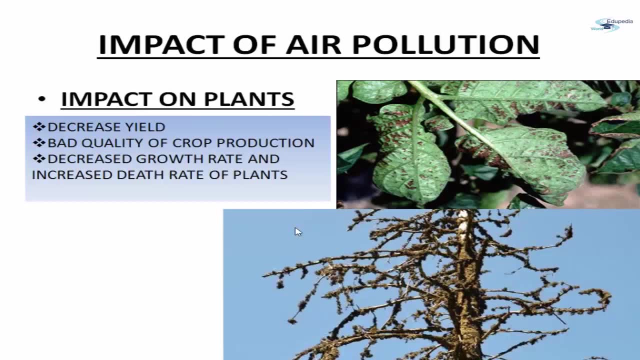 that we are breathing every minute. So if that air itself is polluted, we will have lot of problems in the body. So that is the effect on the human health. Next is impact of plants. So it is not that just the human beings are affected because of the air pollution. 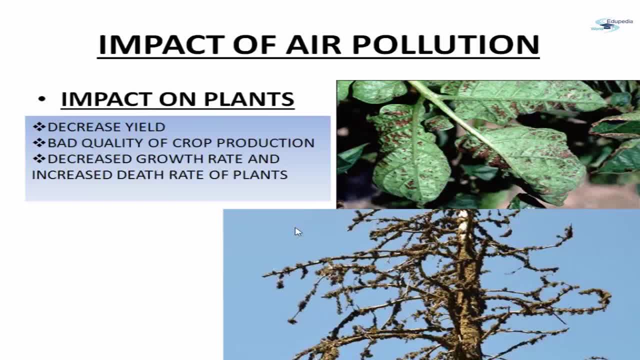 But even the plants are also the same. the plants are also living and these days we take care of the plants as we take care of our children. So the impact on the plants are also the same as there are impacts on the human health Because of air pollution. the quality of the crop will come down. 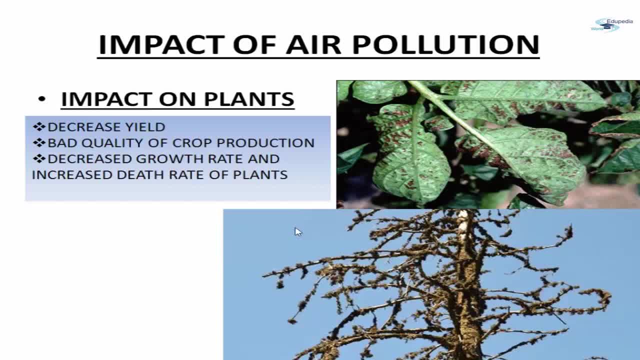 The quality of the leaves that are produced. that will also come down. You see here the leaf. this is all. the leaf is all infected. that is all because of air pollution. The growth of the crop will come down and there will be an increased death rate. 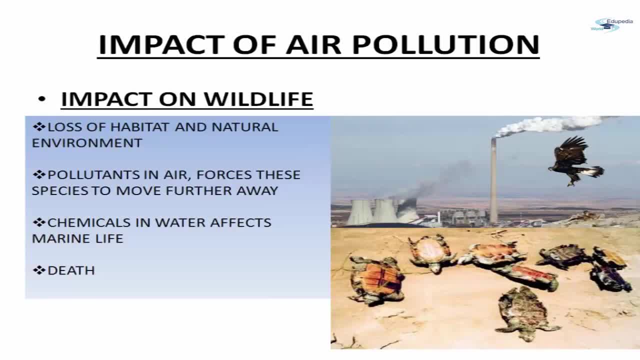 So the impact on mind, life Wildlife are also equally affected because of air pollution, Because of the pollutants in the air, because of pollutants in the soil or in the waters. if there are pollutants everywhere, then these wildlife are forced to move away to a new. 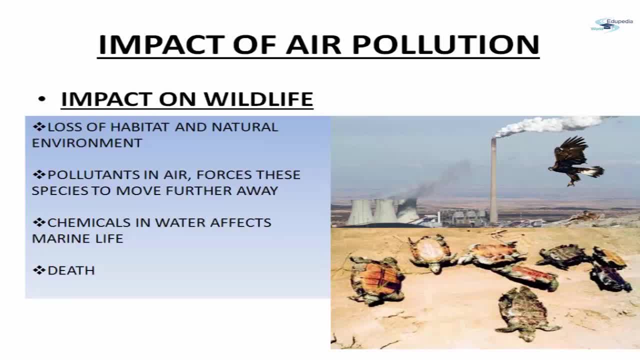 location in order to find pure water and pure air to breathe in. Because of the increase in the air pollution, there are some of the species which have almost come to an end. Increase in the air pollution can also lead to death of the wildlife or other animals. 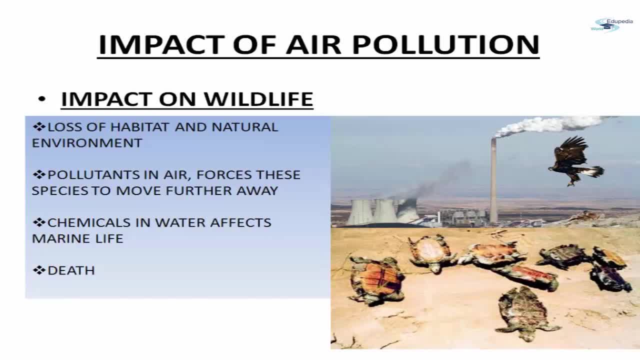 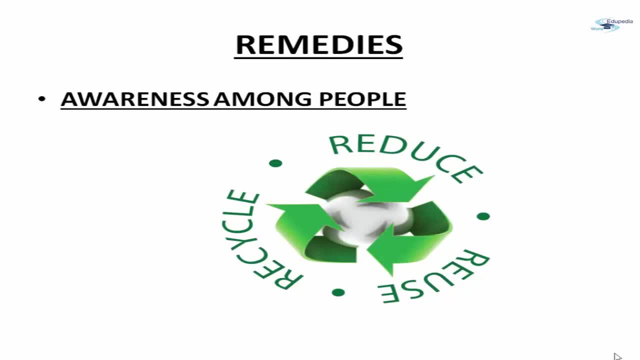 for example, the kettles. So air pollution has an equally dangerous impact on the wildlife. So now that we have talked about the impacts of air pollution, let us also talk about some of the remedies of air pollution. And among the remedies, the first solution that comes up is to make people aware of the 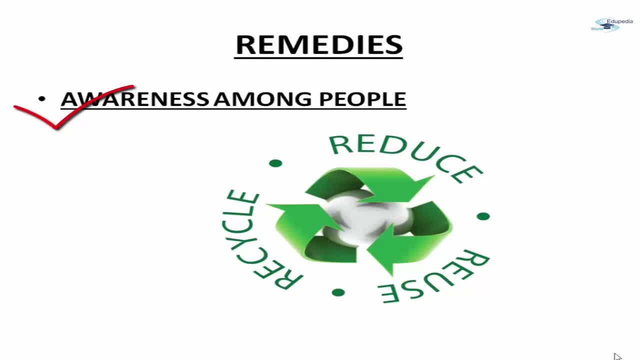 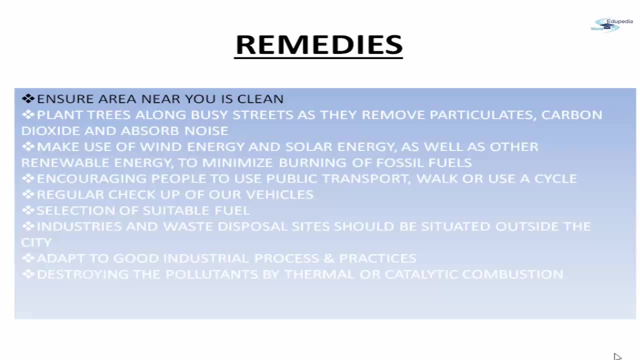 harmful effects of air pollution And also to let them know about the concept of reuse, recycle and reduce, Because only if people are aware of the harmful impacts of air pollution will they take any initiative of reducing this air pollution right. So first and foremost solution is awareness. 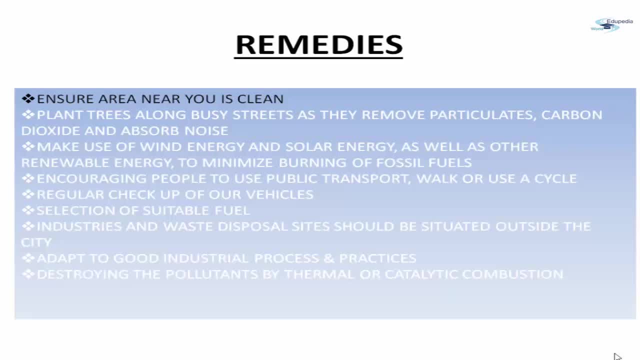 Next to awareness comes to ensure that our area near us is clean. Next is we should grow a lot of plants and trees along the roadside. The trees and plants should be grown in the residential areas so that they absorb the carbon dioxide, so that they absorb the noise. 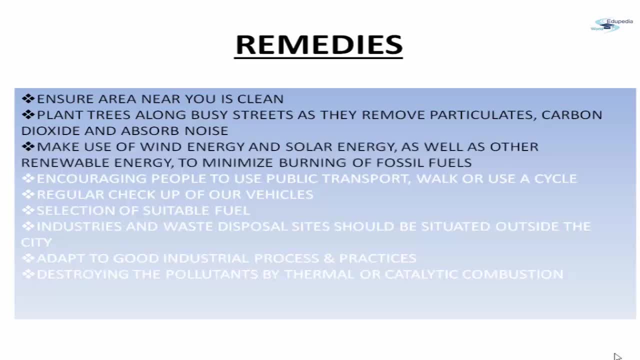 So growing trees is more important. We should make use of wind energy and the solar energy, as well as other renewable source of energy, And we should take efforts in order to reduce this burning of fossil fuel. And how can we reduce the burning of fossil fuel? 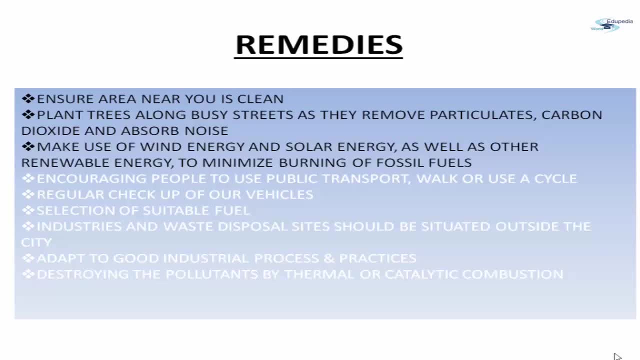 Probably reduce the use of vehicles and we should, as far as possible, use only the natural sources of energy because they are clean. People should be encouraged to use public transport or walk or use their cycles or use some kind of conveyance which will not allow burning of fossil fuel. 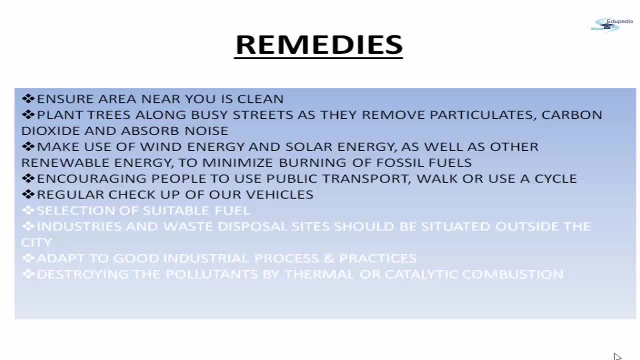 People will use their private vehicles, but what is required is that regular checks of those vehicles need to be done. Next is selection of suitable fuel. Fuel should be selected in such a way that, due to burning of that particular fuel, such harmful gases like carbon monoxide, carbon dioxide- these gases should not be produced. 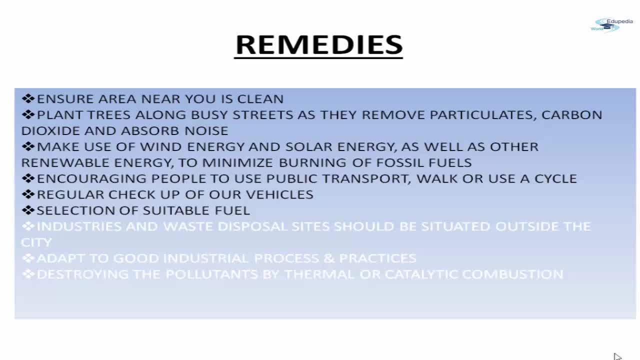 in such large quantity. That's why regular check up of the vehicles is required. Proper selection of the fuel is required. Industries and waste disposal sites should be situated outside the city and away from the residential areas, So that people are away from such dumping zone, such landfills and such sites. 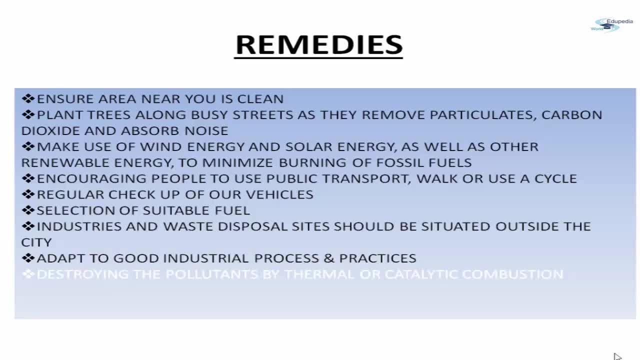 Next is we should adapt to some of the good industrial processes and practices. What do we mean by saying processes and practices is that the industrial process that are taking place should be such a way that there is no release of harmful gases, or even if the harmful 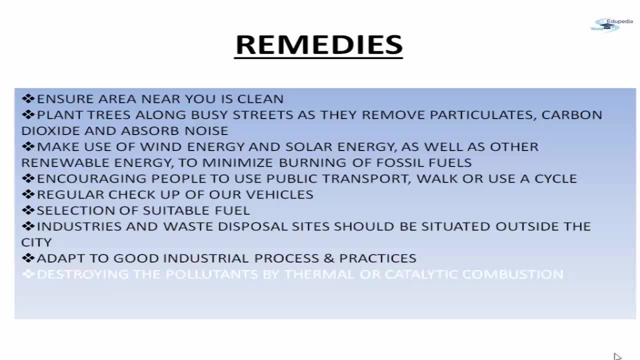 gases are released, then it should be released in very, very lesser quantity. Proper waste management should be planned in order to dump the waste that comes out of the industries, For example, the water, the gases that are released and other solid waste which comes. 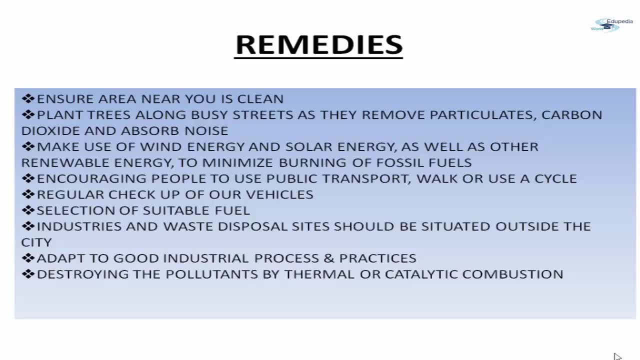 out of the factories and the industry Destroying the pollutant by thermal or catalytic combustion. This is very, very important because by normal combustion if the disposal of the pollutants takes place, then again it will create air pollution. So proper disposal. 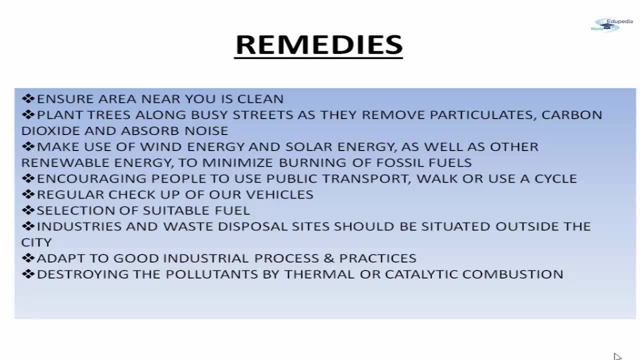 Proposal is required, So for this we should go in for either thermal or catalytic combustion. So these are few of the remedies. Some of the remedies that we spoke about in this session are those which even we as an individual can take initiative right. 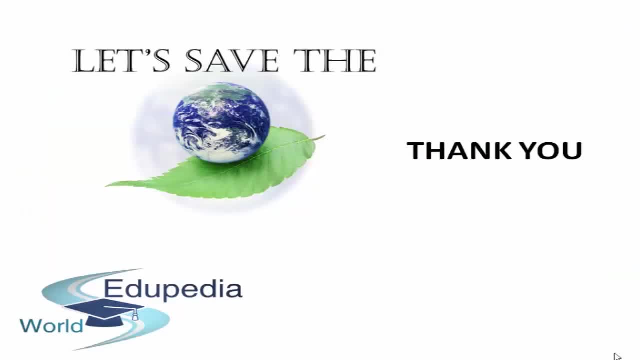 So I hope you must have understood what is air pollution, how the air pollution is caused, what are various manmade and natural sources of air pollution, impacts of air pollution, etc. And finally, what are the probable solution of air pollution. So thank you for watching Edupedia World Videos. 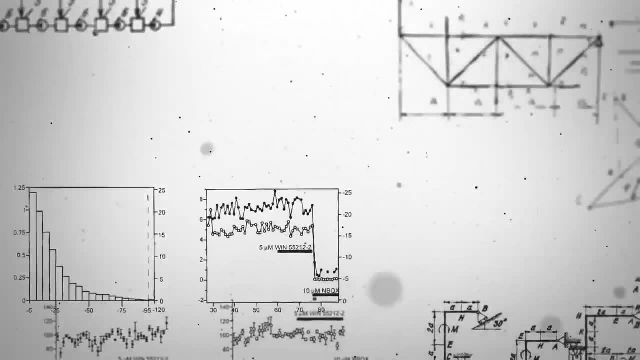 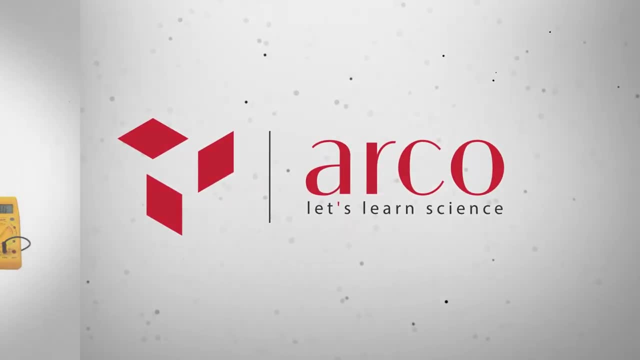 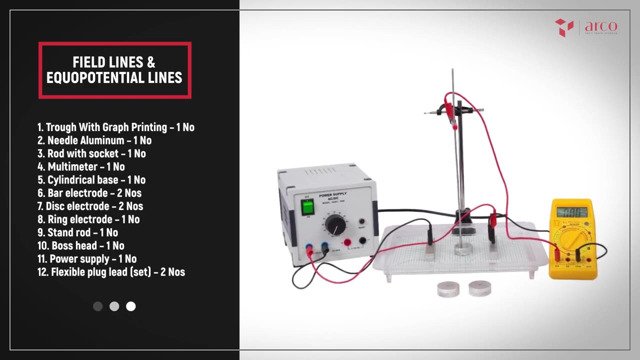 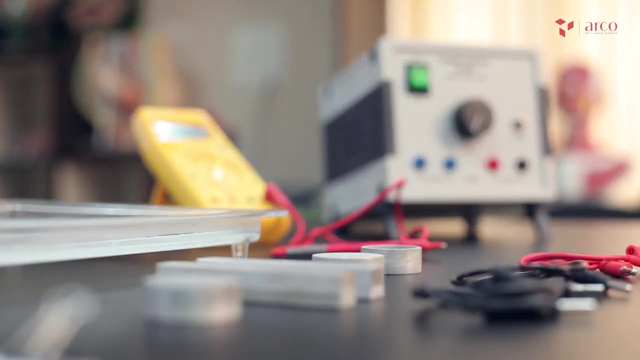 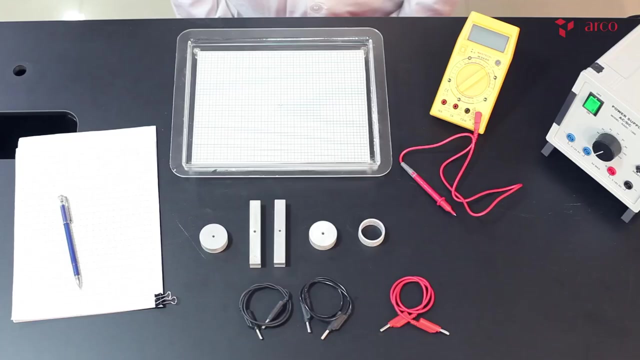 Now we are doing the experiment for field lines and equipotential lines. We will demonstrate about the properties of field lines and equipotential lines. To perform this we need a low voltage power supply, a trough with saline water, 2 bar electrode. You may also use ring electrode. 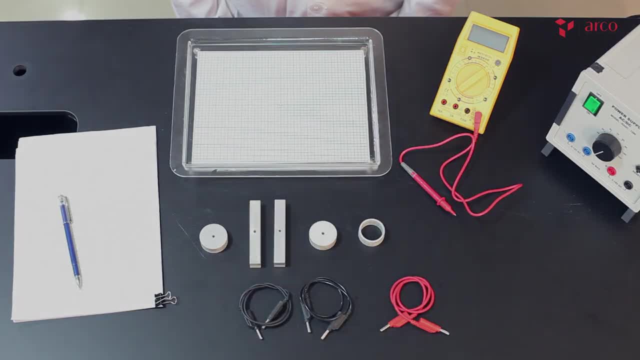 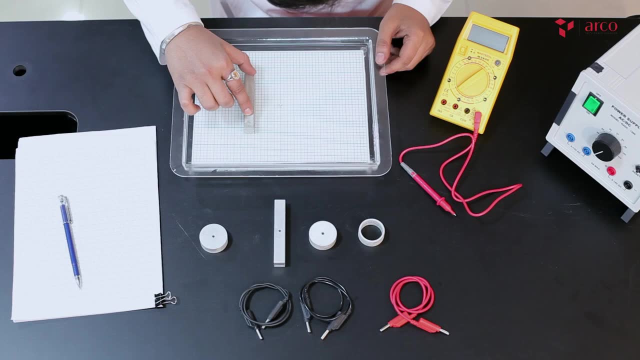 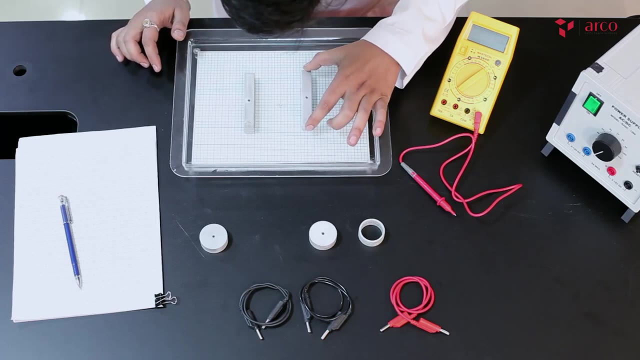 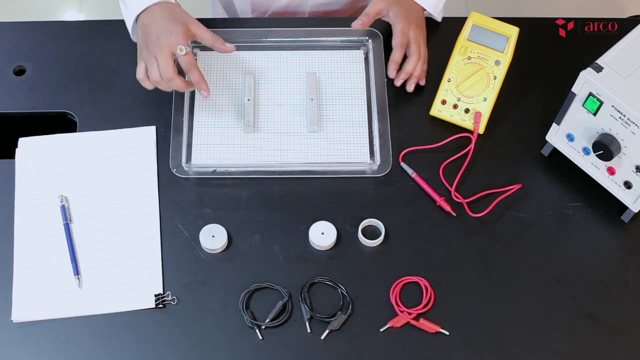 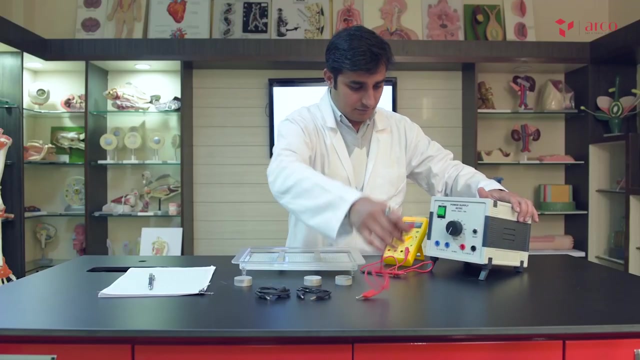 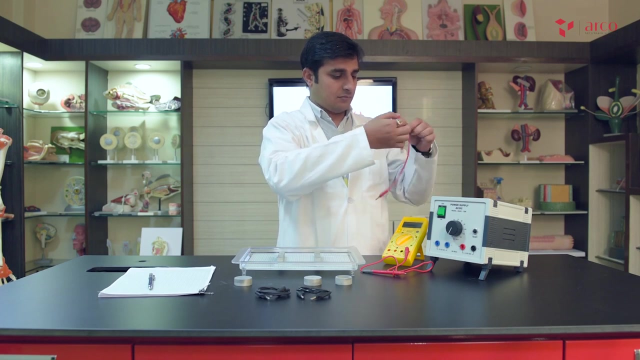 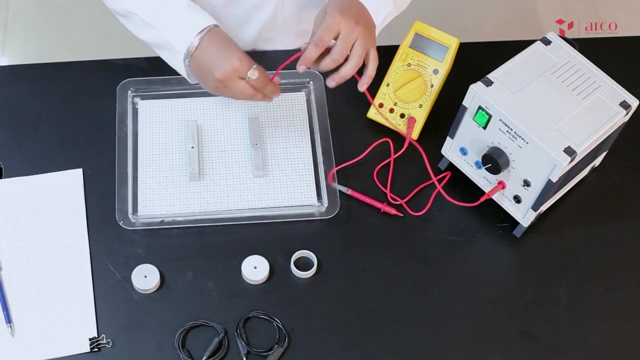 and disc electrode to perform for different kind of fields. Now we will place 2 bar electrode in a trough with saline water And connect the 12 volts DC output to these bar electrodes. So one of the electrode will work as positive electrode and one electrode will work as negative electrode.